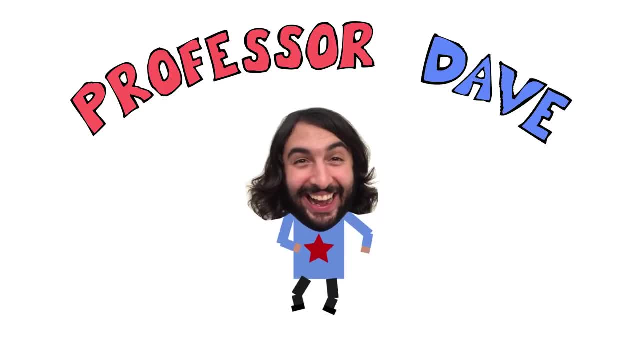 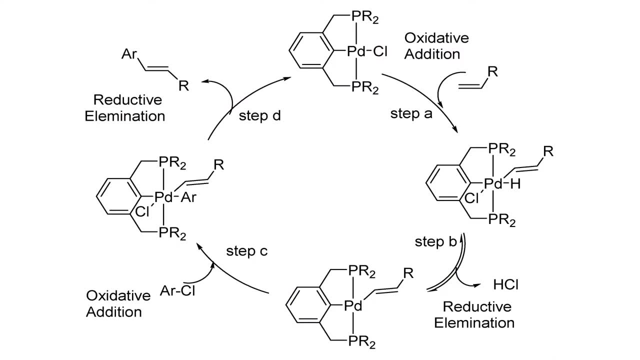 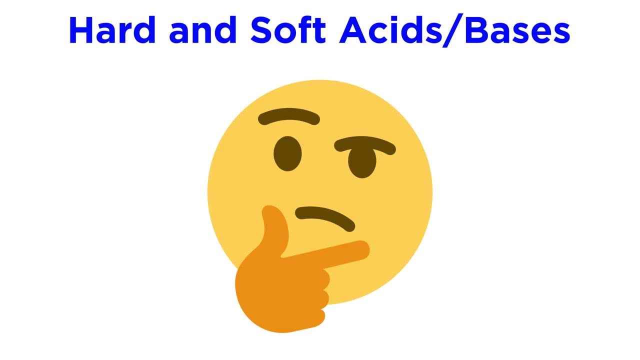 We are almost ready to begin learning about the kinds of chemical reactions that transition metal complexes will participate in. but first let's learn one additional topic that will be of relevance. We must understand hard and soft acids and bases and how they pertain to transition metals. We certainly will recall acid-base reactions from our study of general 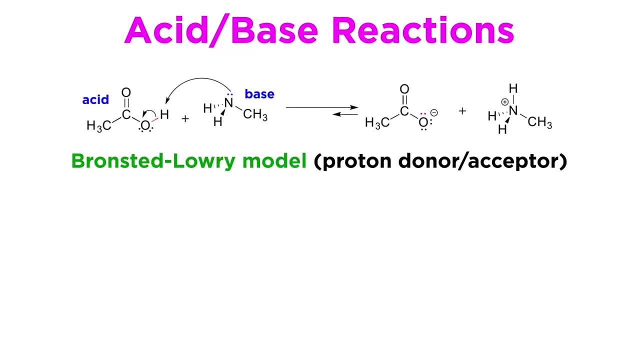 chemistry and we are certainly aware of the Bronsted-Lowry definition for acidity and basicity that deals with proton exchange. But we should also remember the Lewis model of acidity and basicity where a Lewis base is an electron pair donor and a Lewis acid. 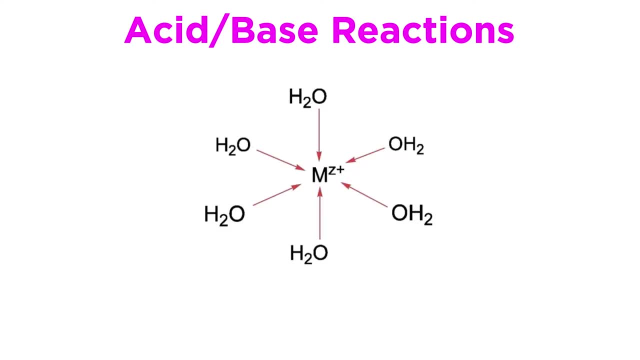 is an electron pair acceptor. This definition will be relevant for us because transition metal centers often act as Lewis acids and ligands act as Lewis bases when they coordinate to the metal centers. So, in the context of this tutorial, when we talk about acids, we are referring to transition. 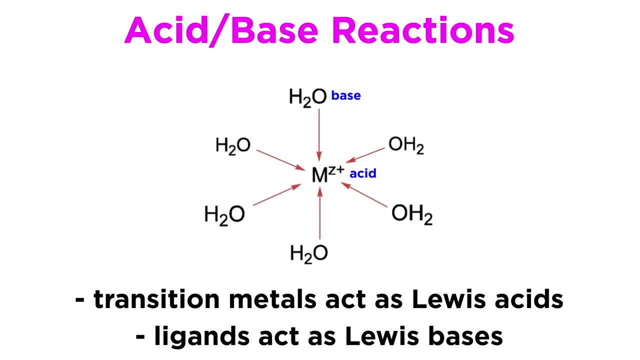 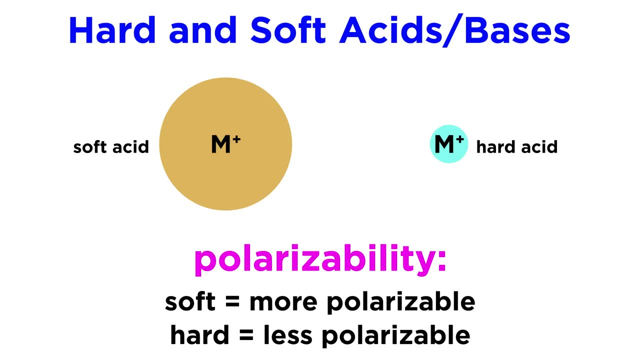 metal ions and bases will be the ligands that coordinate to them. In order to be able to predict the strength of metal-ligand interactions, we need to understand the concept of hard and soft. When we say that an acid or base is soft, we are referring to its polarizability. 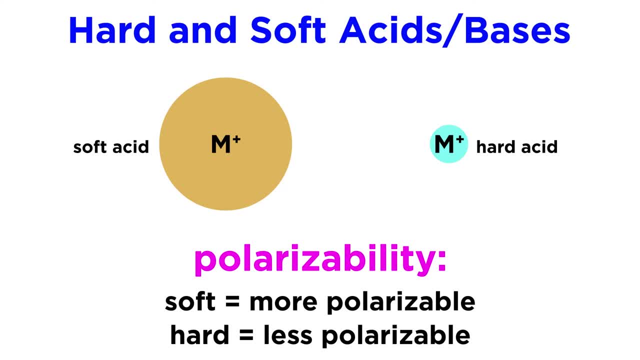 A highly polarizable atom or molecule is very soft. This means that large metal ions are soft. This means that it has a polarizability. So why do we say that these acids are hard? soft acids? They have large electron clouds that can exhibit large momentary or induced dipoles. 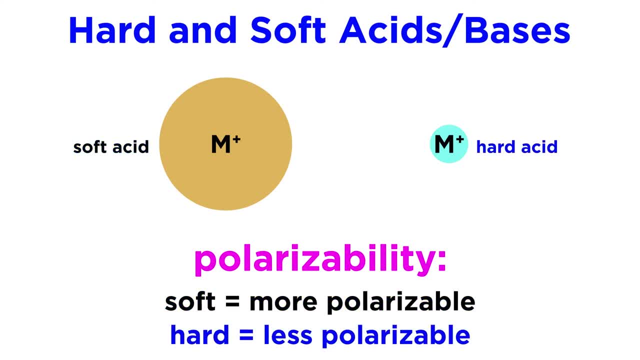 and are thus more polarizable. Smaller metal ions are hard acids. We can say the same for a base. If a lone pair or negative charge is highly localized on a singular small atom, this would be a hard base. If the charge is diffuse, distributed around a larger, 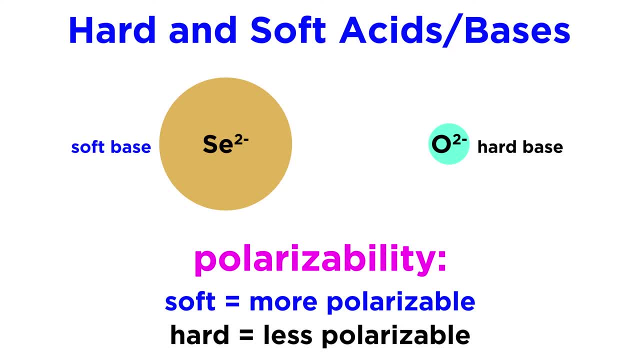 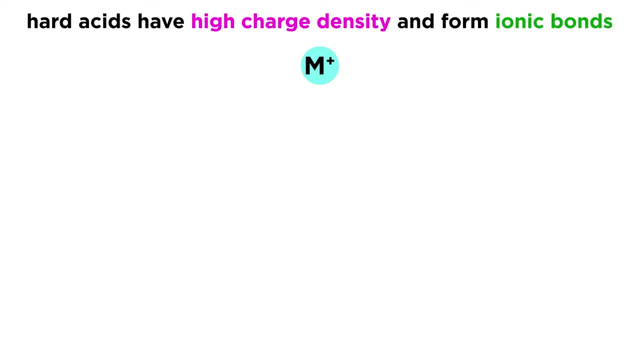 molecular volume or an atom with a large radius. this would be a soft base. Hard acids have a high charge density and form bonds that are more ionic in nature. The greater the charge on a metal ion, the harder it is, and the smaller the radius of the metal ion is, the harder it is. 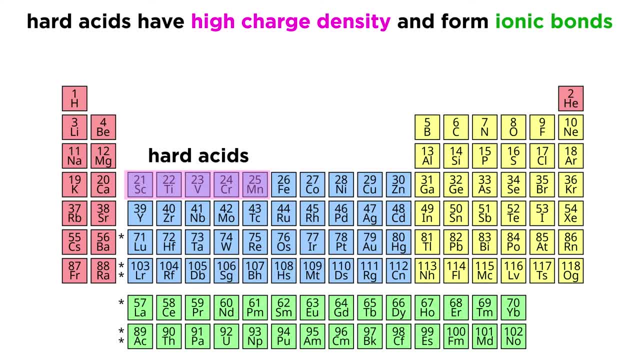 Early transition metals with valence electrons in the 3D subshell are hard acids. Hard bases are small anions which are hard acids. Hard bases are small anions which are hard acids. Hard bases are active and neutral molecules with lone pairs. Bases derived from electronegative 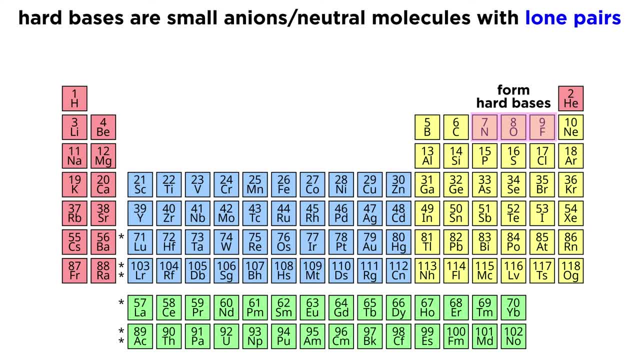 elements in the N equals two shell will be hard bases like those of nitrogen oxygen and fluorine. This means that fluoride anions, any kind of oxygen anion like an oxide or a hydroxide, and even neutral nitrogen atoms in ammonia or other amines are classified as hard. 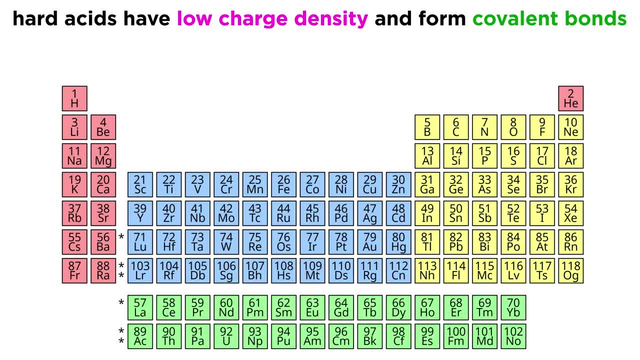 Soft acids have a lower charge, density and form bonds that are more covalent in nature. Late 4D and 5D transition metals tend to be soft due to their larger size and polarizability. These usually have charges of only 1 plus or 2 plus. Soft bases are larger anions and 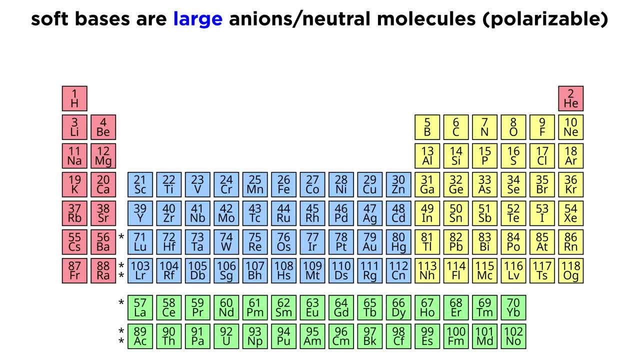 neutral molecules which are more polarizable than their hard counterparts. For example, while fluoride is hard, iodide is very soft and the softness increases going down the halogen group as radius increases. Likewise, while an oxide ion is hard, a sulfide ion is much softer. 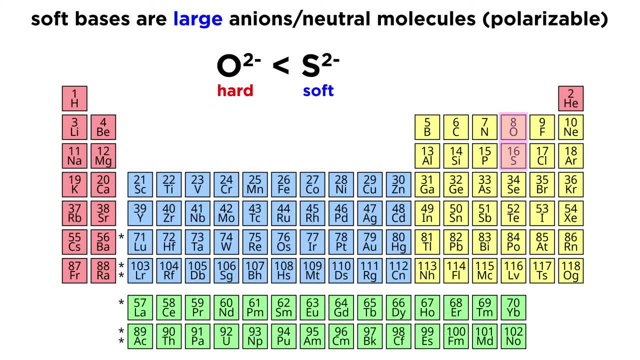 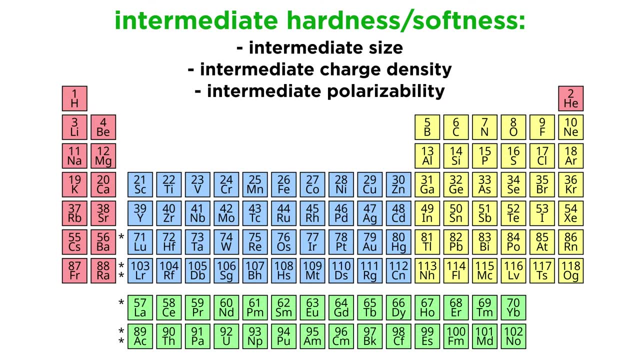 again due to the increased radius and polarizability. There are also plenty of species that qualify as having intermediate hardness or softness, not leaning heavily in either direction. These have intermediate size, charge, density and polarizability. This is not always easy to predict, as even different oxidation states of the same element 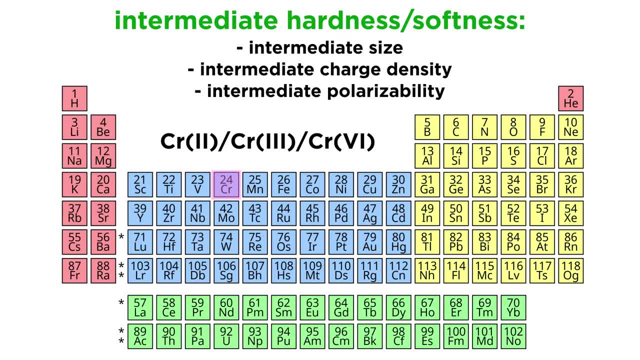 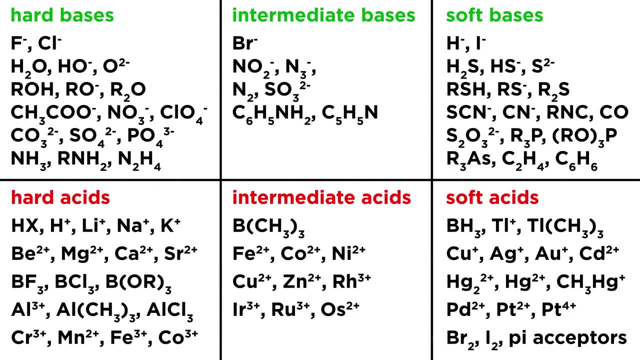 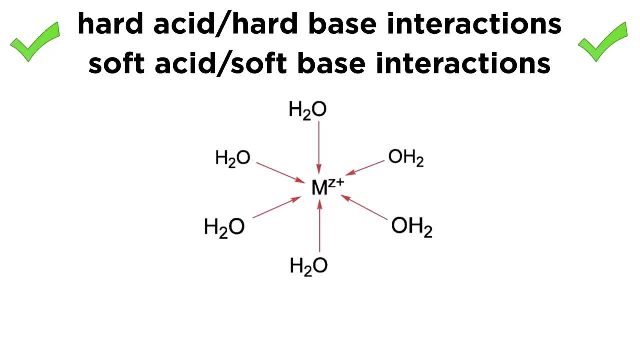 can differ dramatically, so it is best to just learn through example as we go through the series. But for those who like to get a glance at the bigger picture, here is a table depicting some common hard and soft acids and bases. The key thing we must understand when applying this framework to metal-ligand interactions. 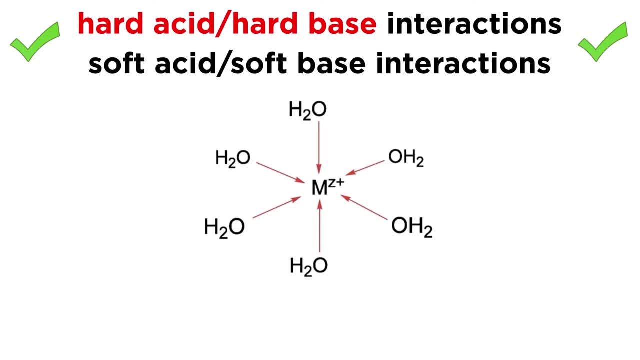 is that hard acids interact best with hard bases and soft acids interact best with soft bases. This means that hard acids interact best with soft bases and soft acids interact best with soft bases. This means that the stability of a complex is enhanced by hard-hard and soft-soft interactions. 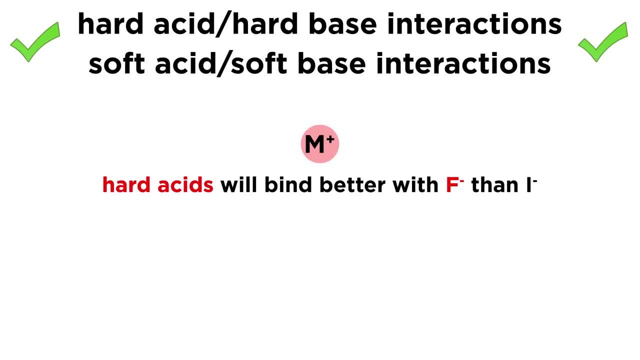 so a metal center that would be regarded as a hard acid will bind better with fluoride than iodide, and for a soft acid that trend would be reversed. This phenomenon can help us understand and predict the types of complexes a metal center will form. Take a very soft acid like gold 1+. This will only